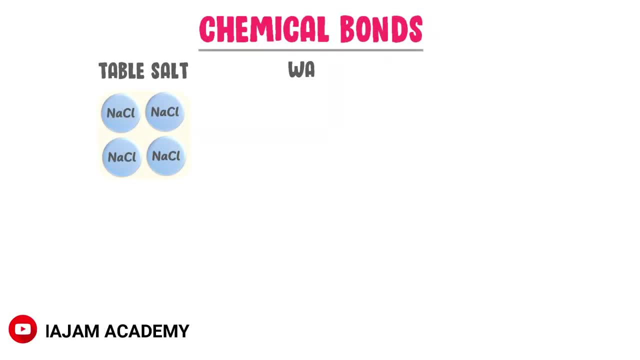 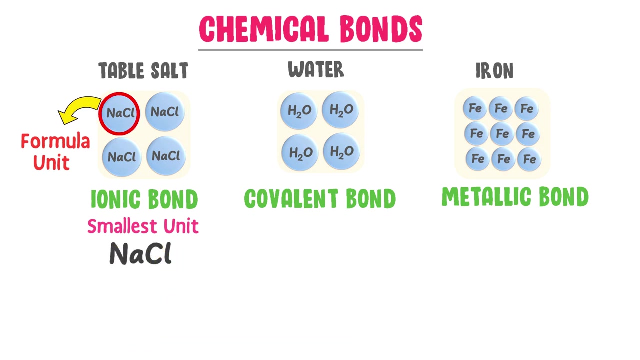 of chemical bonds. Consider table salt, water and pure iron sheet. We know that table salt contains ionic bond, water contains covalent bond and iron sheet contains metallic bond. The smallest unit of ionic compound is formula unit, like NaCl. Ionic bond is formed when sodium loses one electron. 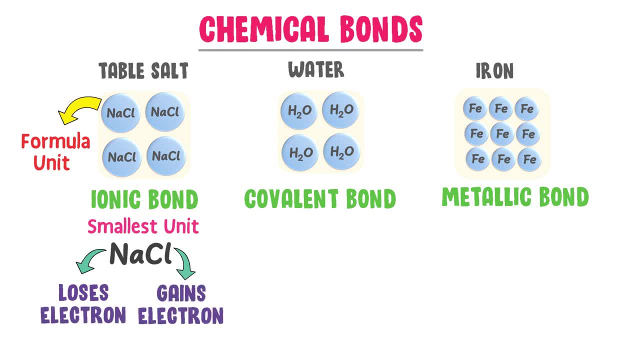 and chlorine gains one electron. As a result of this, a single formula unit of table salt is formed, like NaCl. Hence we say that all sodium and chlorine atoms in the table salt are joined together by losing and gaining of electrons. Now the smallest unit of covalent bond is: 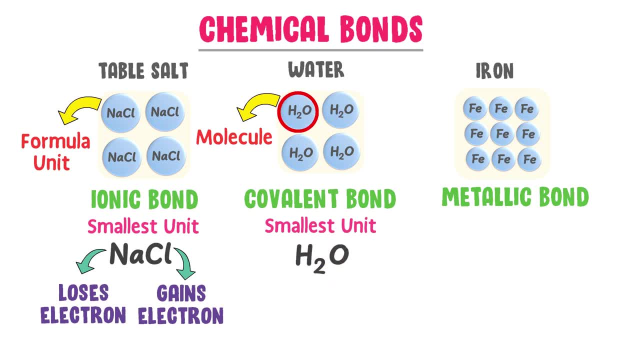 a molecule like H2O. Covalent bond is formed when oxygen atoms shear its two electrons with each hydrogen atom. As a result of this mutual shearing of electrons, a single molecule of water is formed. hence, all these water molecules are joined together. 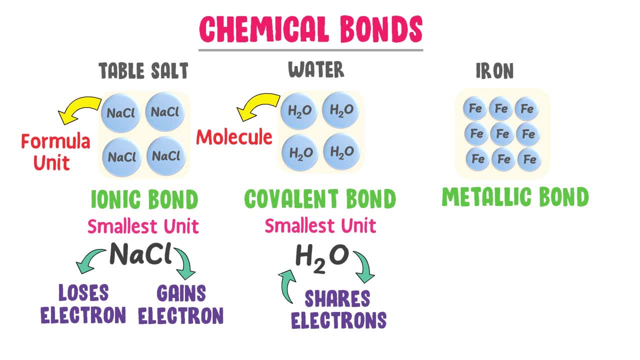 due to covalent bond. therefore, remember that ionic bond is formed by transferring of electrons and covalent bond is formed by mutual sharing of electrons. now, in the metallic bond, the smallest unit is an atom like this iron atom. metallic bond is neither formed by transferring of electrons. 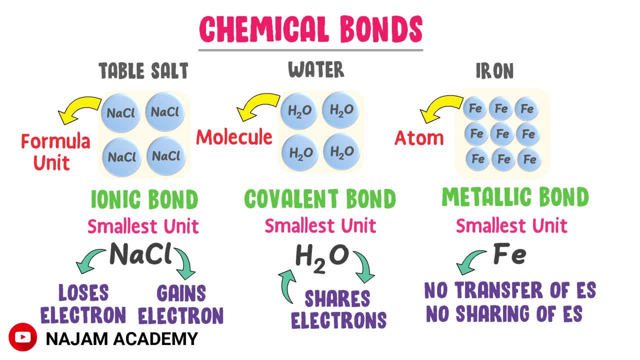 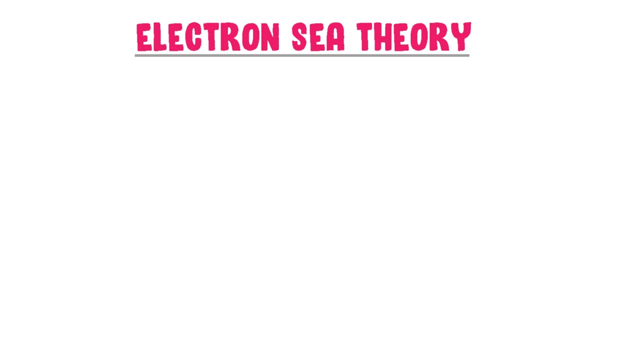 nor by mutual sharing of electrons. then how these all iron atoms are joined together chemically? well, there are different theories that explain the metallic bonding, but the most common is electron c theory or electron gas theory. let's consider a pure iron sheet. according to electron c or gas theory, this single atom of iron will lose its two valence. 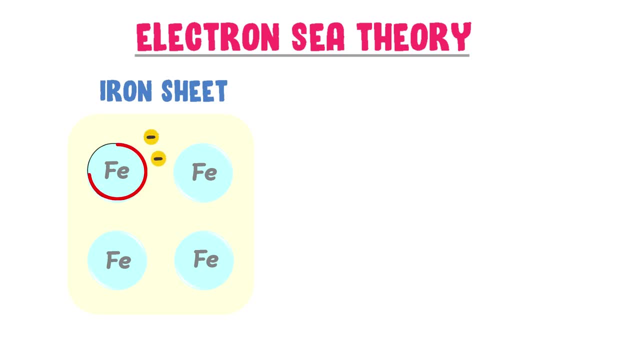 electrons within the sheet. the iron atom has lost its two valence electrons and will become double positively charged. similarly, this iron atom will lose its two valence electron and will become double positively charged. this iron atom will also lose its two valence electron and will become double positively charged. this process of losing valence 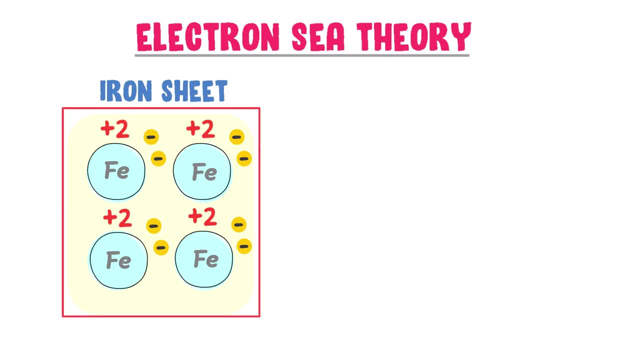 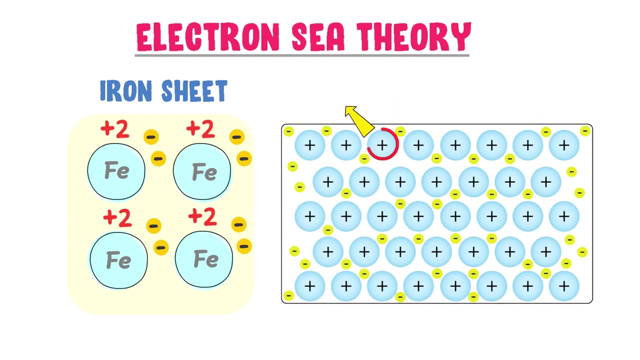 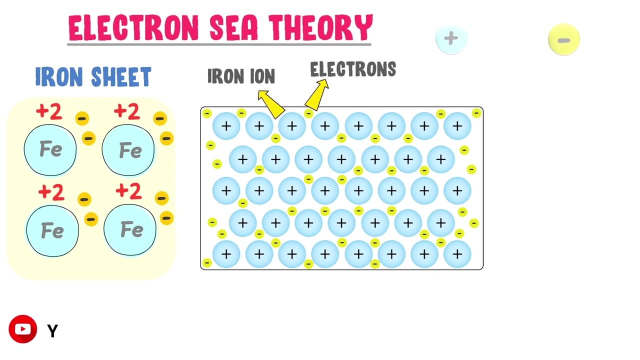 electrons would continue until all the atoms of iron sheet will lose their valence electrons and will become positive ions. so the structure of iron sheet will be like this: after losing electrons, the positive charge you see is the ion of iron and all these lost electrons will form a sea of electrons or clouds of electrons around these positive ions. we know that positive. 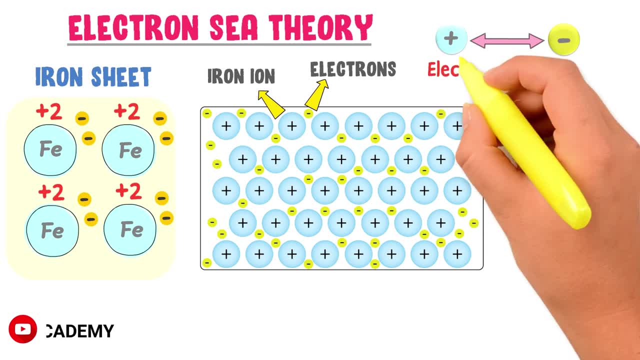 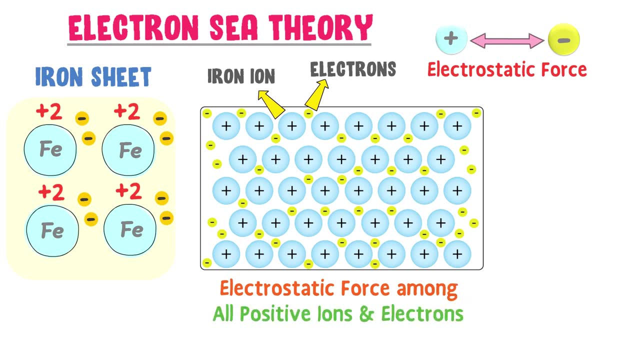 and negative charges attract each other due to electrostatic force. hence, there is electrostatic force among all positive ions of iron and the sea of electrons. let me repeat it: there is electrostatic force among all positive ions of iron and the sea of electrons. this electrostatic force acts as a 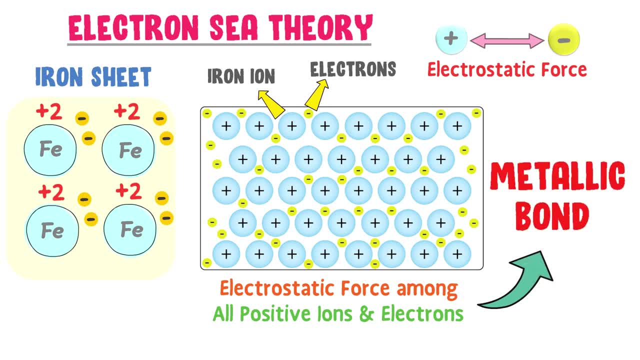 metallic bond and hold together all the atoms of iron. noted down that these lost electrons do not belong to any individual atom. rather they form a cloud or sea of electrons and the letters- secondly, these electrons are called delocalized electron because they move freely within the iron sheet- are letters, so they are also good conductor of heat. 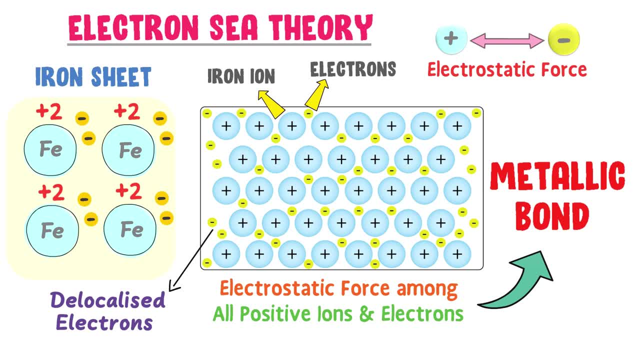 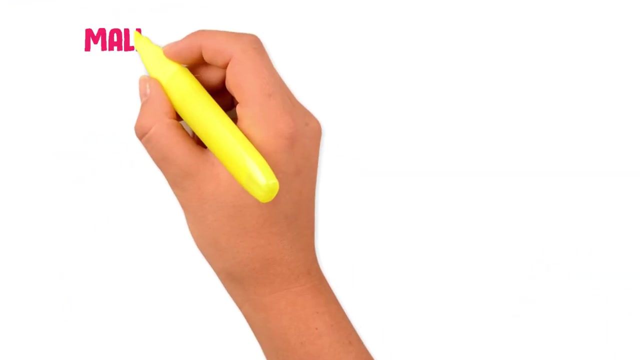 and electricity due to free electrons. metallic bond exists in all metals like zinc, copper, gold, etc. therefore, remember that metallic bond is formed due to the electrostatic force between sea of electrons and positive ions. finally, let me repeat it. teach you that why metals are called malleable and ductile. well, malleability of metal means. 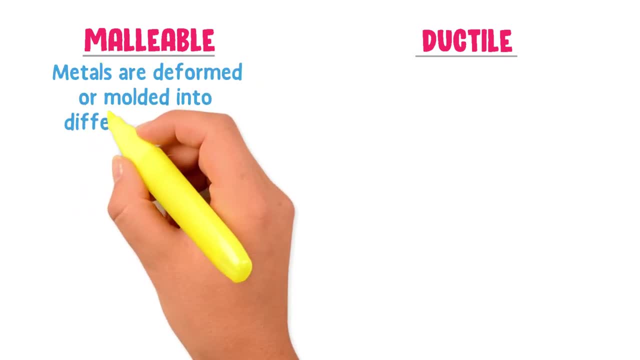 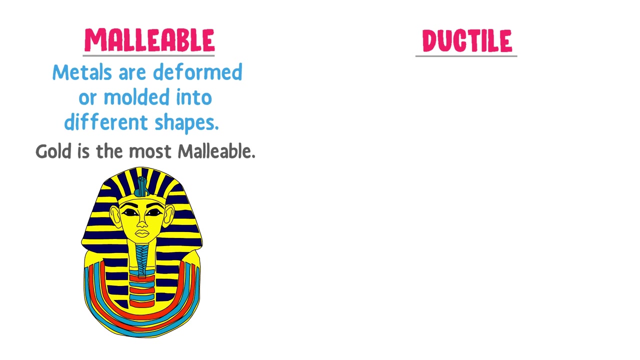 that they can be deformed, are molded into different shapes. for example, gold is the most malleable metal. it can be transformed into different jewelries. this property of metal is called malleability. secondly, ductility of metals mean that they can be drawn into wires.